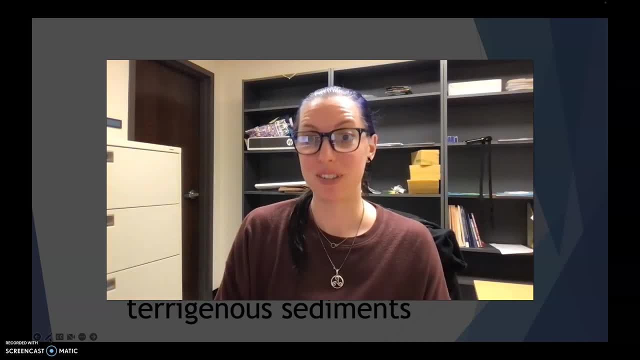 All righty, welcome back, friends. So for this next segment we are going to focus on the origin stories of the different types of sediments. So we're talking about the origin stories. There's four main ones: Lithogenous, which means of the land, Think of like the lithosphere, right. So 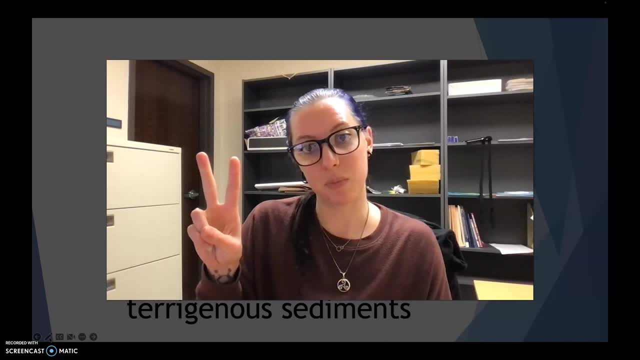 similar sort of root word there, And we have biogenous, which means they're made out of biological things, so living things of sorts, And then hydrogenous simply means chemical reaction. So the ocean is extremely corrosive and it can do some chemical damage. 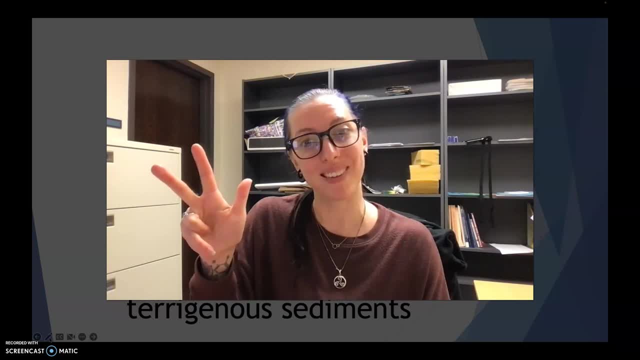 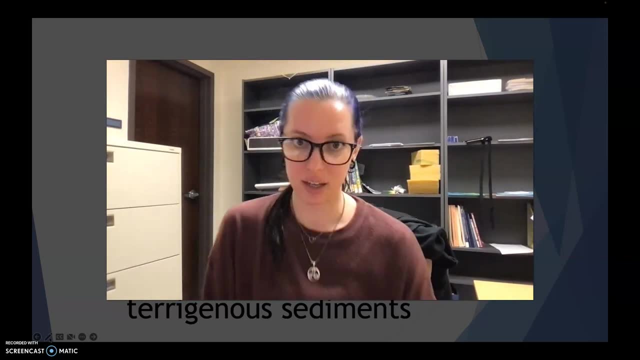 Not. maybe not damage is the right word, but do some chemical reactions. And then, lastly, is cosmogenous. So I want you to first think when we think of where sediments come from, in terms of from the land. think to yourself, maybe pause the video for just a second. 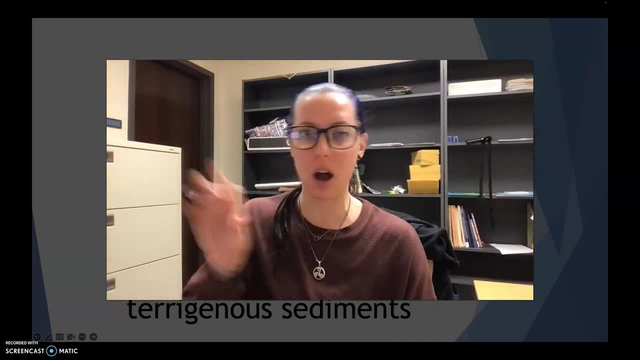 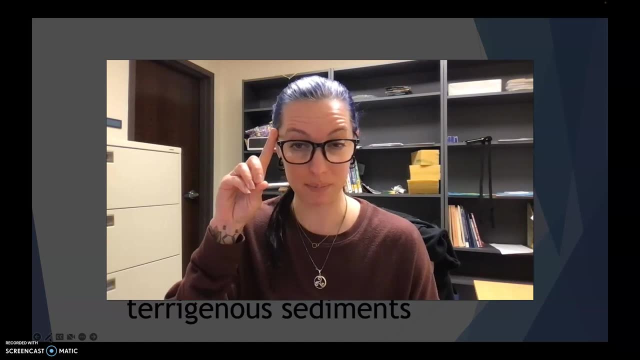 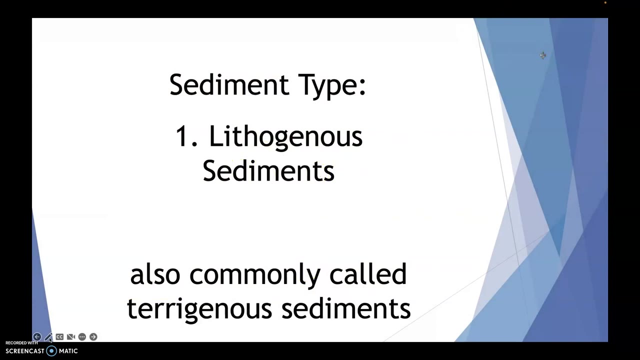 and think to yourself where these could come from. Where on earth could these things come from? So think about it, Think about it, Think about it. Okay, So of the land. And, by the way, lithogenous can also be known as torogenous. Those two words are interchangeable. 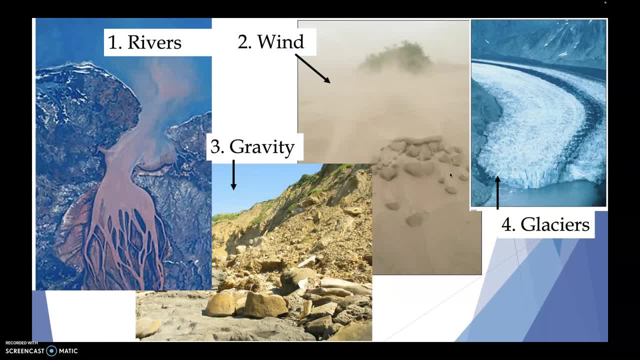 So the four main ways that we can get lithogenous sediment, one to be from rivers right. We've seen a couple of examples already this semester of rivers flowing into an area, into the oceans, And we can literally see a browner, murkier color. 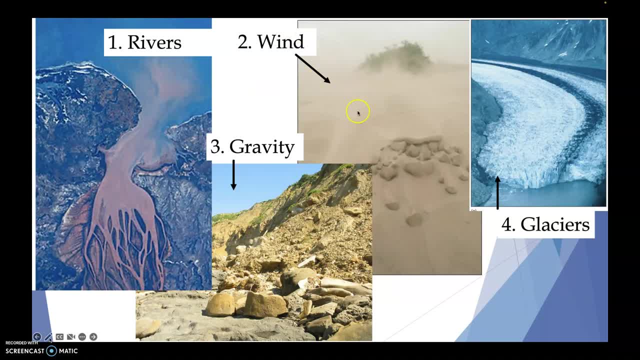 as opposed to out in the open ocean. The wind is also an extremely good mover of dust and those finer sediments. We oftentimes see huge dust blooms off of big, big, big deserts like the Sahara Desert, And we can literally see a huge dust bloom off of big, big, big deserts like the. 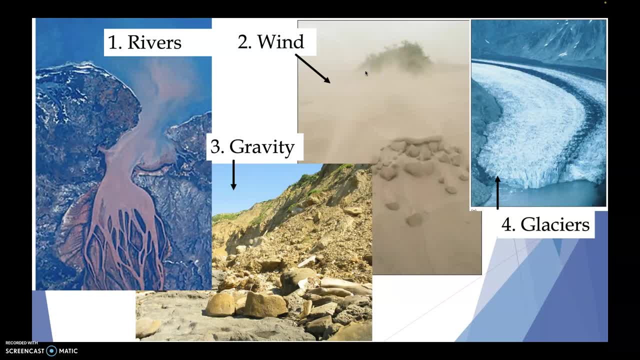 Sahara Desert in Africa, in Northern Africa, And those are blow over into the Atlantic Ocean and actually settle onto the surface of the ocean, which actually ends up being good nutrients for phytoplankton, But we'll talk more about that later. Wind also is a really dang good eroder. 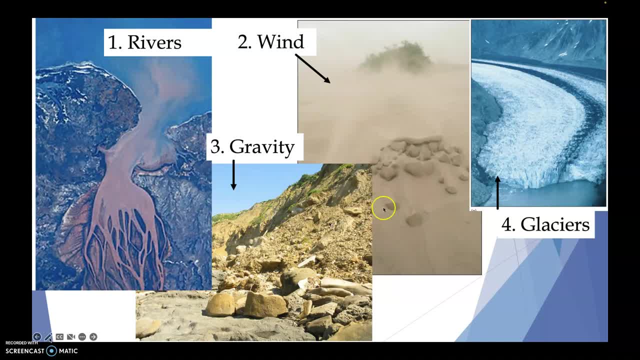 as well, So with wind and gravity, can come into this term of erosion, So the breaking down of the the harder sort of rocks that are right next to the shore, And also- and this is one is kind of often forgotten, I think- 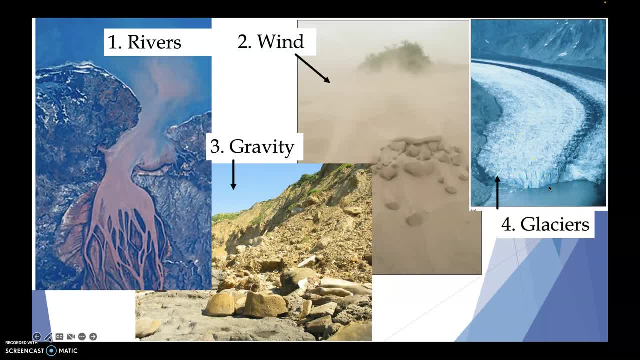 is that of glaciers, So ice is an extremely efficient mover of land. Things get carved out by ice all the time. Think of like the Great Lakes of the Northern United States. Those were carved out because of glacial activity And a lot of like how the Great Plains. are also these really beautiful? 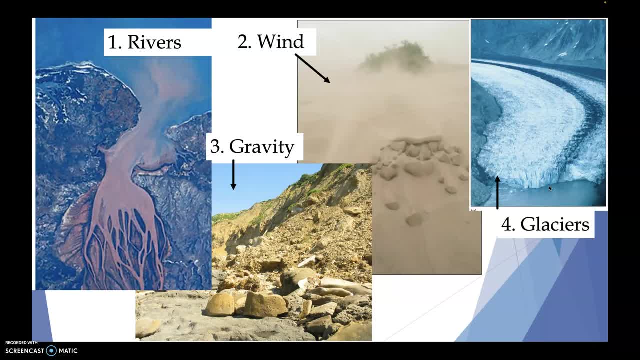 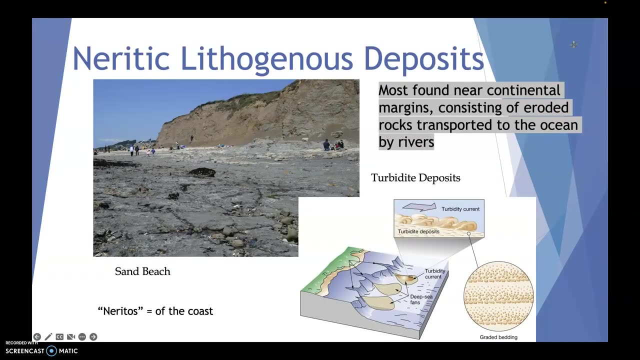 rolling hills And those were likely formed from the movement of glaciers. So there's kind of- excuse me, two, two like further classifications of different types of lithogenous sediment. The first is called narratic lithogenous deposits, So narratic means of the coast. So these would be. 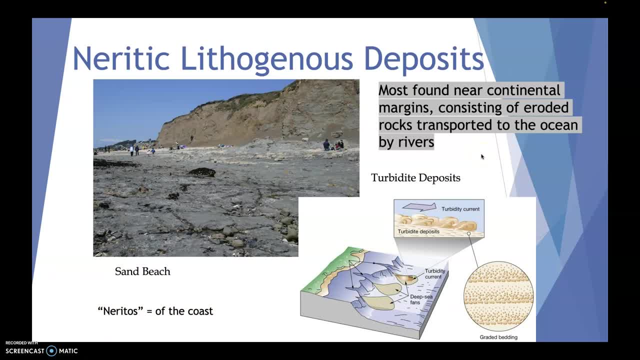 more like. they're found closer to the continental margins And they usually consist mostly of a eroded rocks that are that are transported to the ocean by rivers, And I also have going back to this idea of turbidite deposits. right, we talked about those deep sea fans and how river currents can kind. 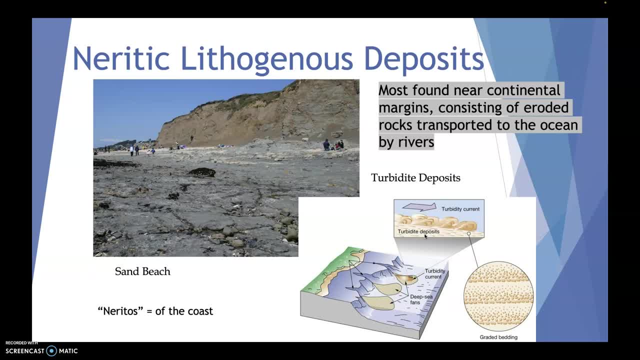 of churn things up a little bit And it gives it this really beautiful sort of swirly kind of pattern and the conventionally settled down And then we'll see some graded bedding in that. I'm hoping to have a video made in the next several days or so of a demonstration that I have at one of the other schools here. So narratic. 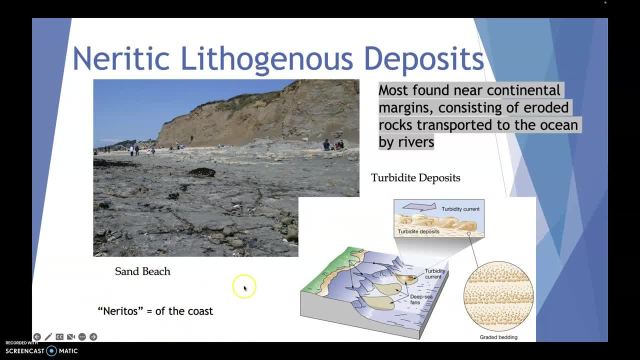 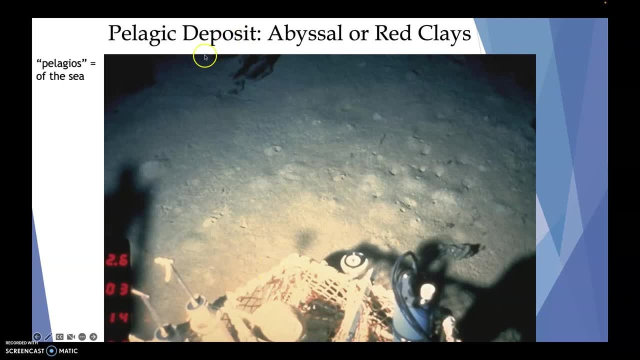 lithogenous deposits simply means of the coast or of the land. Alternatively, we have another term for the deeper oceans and this is called pelagic deposit, So abyssal, or red clays. So pelagios means of the sea. So as opposed to coming from the land, 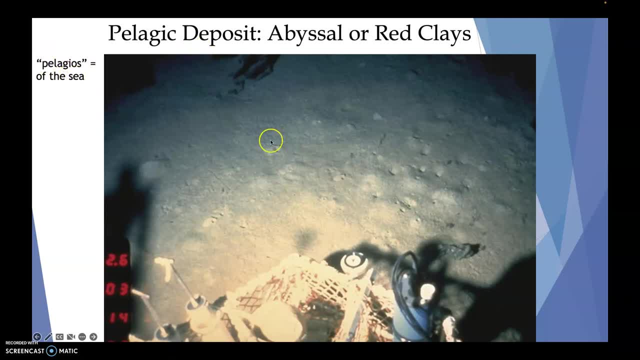 necessarily we're coming from the sea Again, this, this, this image here kind of gives me like a really sort of like if you were to stick your hand in it, it would like give like a really kind of nasty, like I don't know noise. 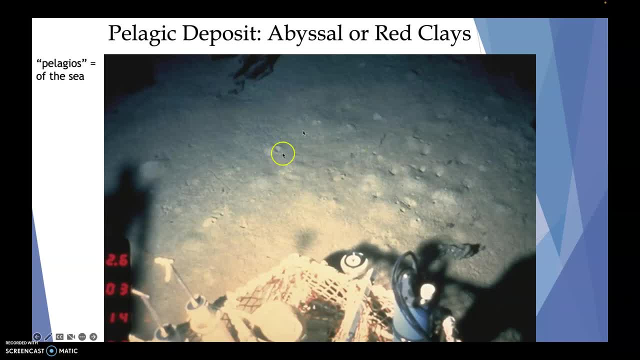 Just how kind of smooth it looks right And also consider how kind of very smooth, maybe a little bit dimply here and there, but overall a very kind of flat sort of pattern here. And a really good exercise to do which may be beneficial is to look at the different thicknesses between the narratic versus pelagic deposits of lithogenous deposits. 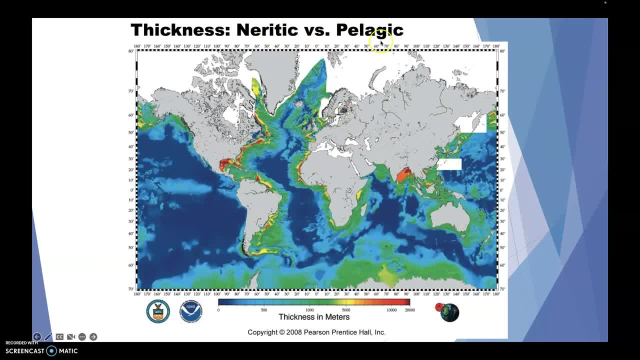 So this here is a map looking at narratic versus pelagic deposits: the warmer colors indicating a thicker deposit or thicker thickness, and the cooler colors indicating a cooler color, cooler thickness. So what I would suggest you do is pause the video real quick or at the very end. 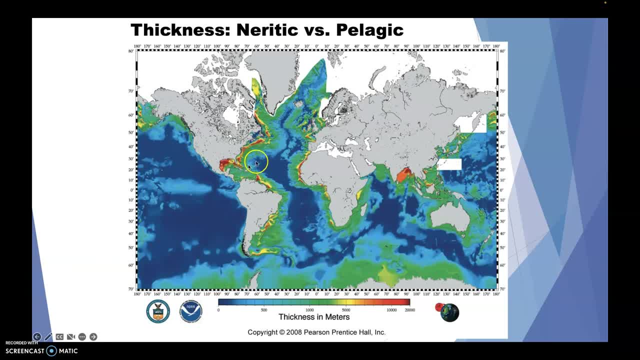 when you're looking over the slides, consider where you see some of these thicker thicknesses of these deposits, of these sediment deposits, before we hit rock right, Right along the coast lines. right is where we see the greater thicknesses of these deposits. So it's a really 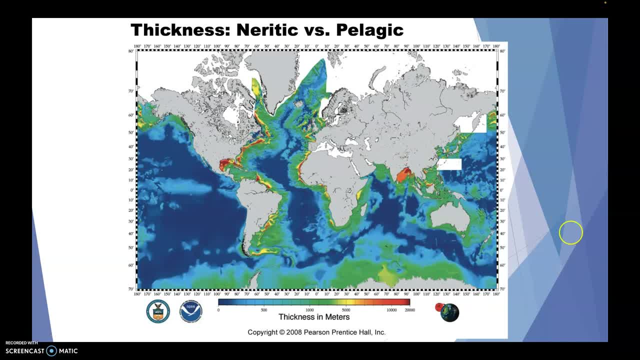 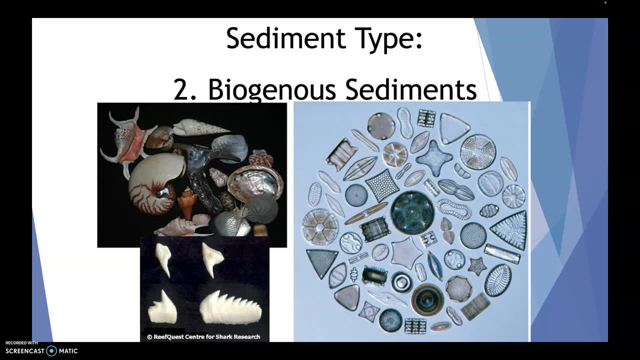 interesting thing to point out. Our next type of sediment is biogenous sediment. So biogenous, think of biology, meaning you know, of life, of some sort of living thing that can consist of a variety of different shells or, like sand, dollars or creatures or skeletons. This picture: 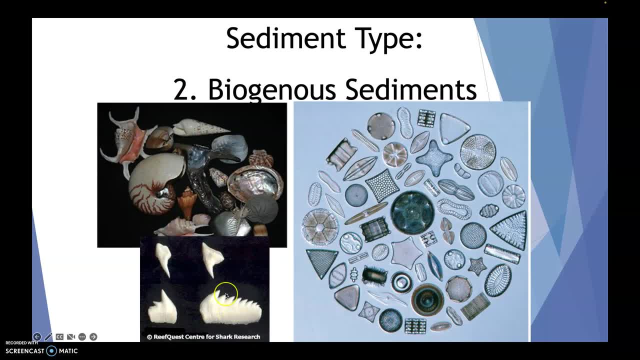 here is just showing all the different kinds of shells that are out there, or bones or teeth. right, Lots of sharks have lots of teeth And they fall out and they're going to end up somewhere. They'll usually end up at the bottom. 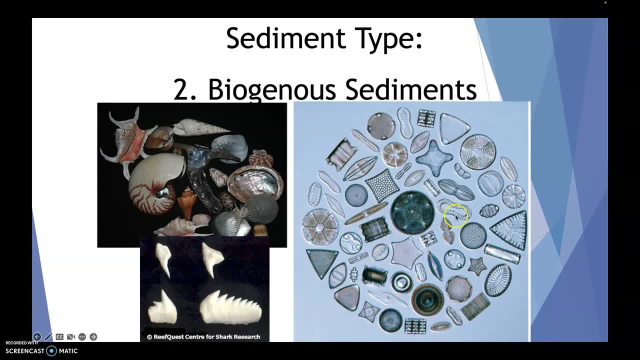 of the ocean, Or this image here on the right side are different types of plankton. We'll talk much deeper about plankton later on, but I just want to kind of point out, just to check out, how symmetrical these creatures are. They're microscopic. You cannot see them with your 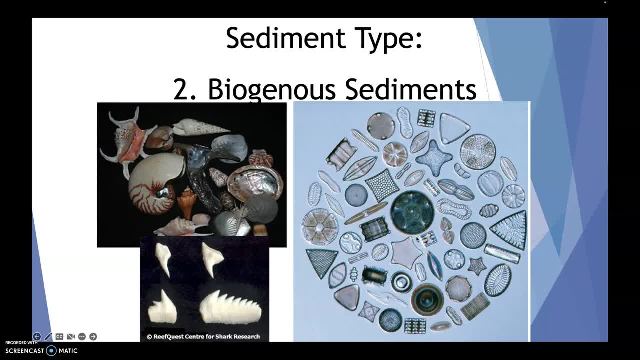 naked eye, But just the fact that Mother Nature can make something so pretty and so small and so symmetrical is really, really quite fascinating. Another thing I want to talk about is the fact that we have so many different types of creatures and so many different animals that we're actually gonna create a bio-genesis. settlement system, And so we're gonna have to figure out how to make a biogonous settlement system, And the first thing that we have to consider when we think of biogonous sediments is poop is gonna be involved in this as well- Lots of whale poop, These big creatures gotta. take big poops as well as- and that's gonna be, you know, broken-down plankton or some of the creatures that eat meat, Like some of the killer whales or dolphins. Their poop is gonna consist of, you know, bits and pieces of the animals that they've consumed. I know. 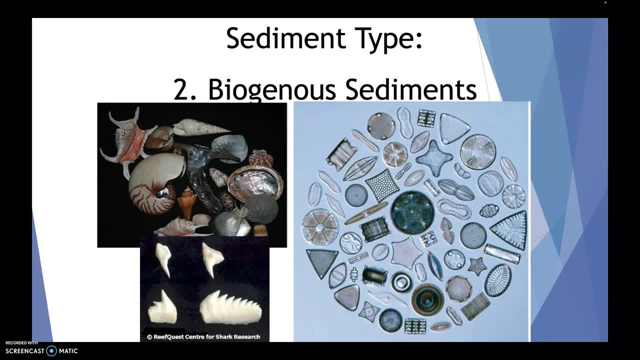 that sounds really gross, but it's just the reality of Mother Nature. So we're gonna have to figure out how to make a bio-genesis sediment system. And then These big creatures got to take big poops as well as- and that's going to be, you know, broken down plankton or some of the creatures that eat meat, like some of like the killer whales or dolphins. their poop is going to consist of, you know, bits and pieces of the animals that they've consumed. 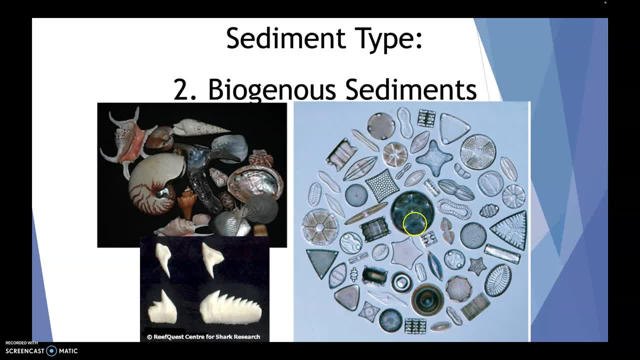 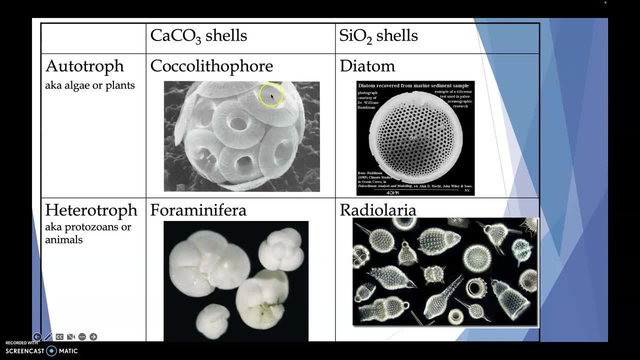 I know that sounds really gross, but it's just the reality of Mother Nature. But first we're going to talk a little bit further on this idea of plankton. So there's two kind of different shells that we observe with different plankton. 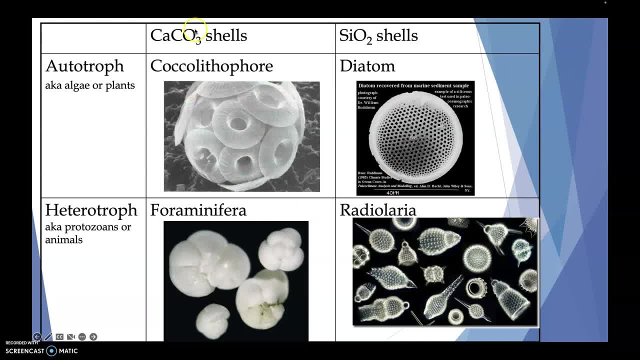 Right now we're going to focus on four different kinds of plankton and kind of broken down into separate varietals. So on the top row here we're looking at autotroph plankton, meaning that they are algae or plants, meaning they make their own food. 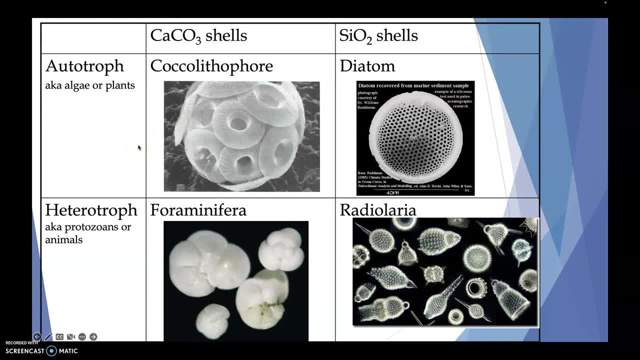 They make their own food. They don't have to eat anything else. in order to sustain, They use the sunlight and they use carbon dioxide and they take that and that's their energy. The second row are heterotrophs. So heterotroph means that they are some sort of protozoan or animal, meaning they have to eat other animals in order to sustain life. 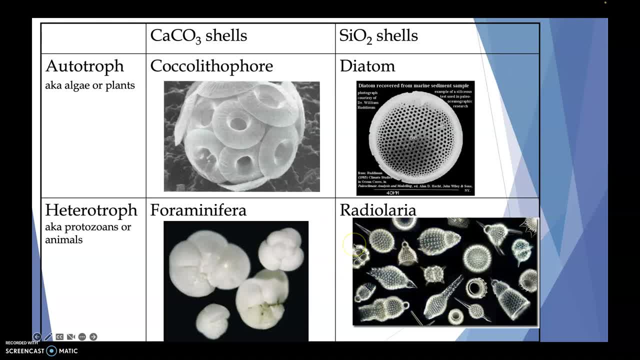 So they can't just hang out in the sun and call it a day. They actually have to physically eat other things From there. we can also break them down into chemical composition. So the CAC, CACO3. That just means calcium in a way. 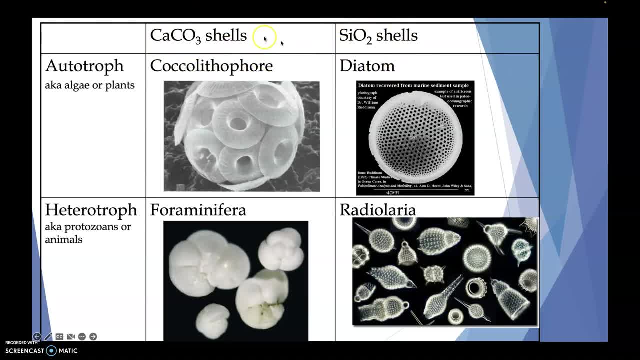 Calcium carbonate shells versus silicon shells. So calcium carbonate versus silicon. As you can imagine, one requires calcium Like. calcium is good for our bones, right, We need to drink all the milk so that our bones grow big and strong, Whereas silicon and this one's going to be a little bit of a weird analogy, but if anyone gets any sort of breast augmentation, 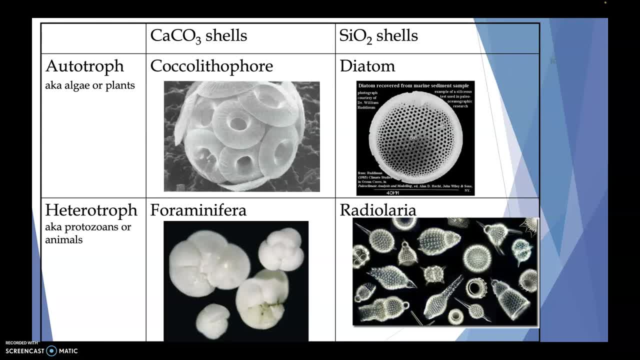 fake boobs are made out of. So it's kind of a way to think of it that way. But when we break down these different sediments, we can kind of further break them down in this way: Are they made out of calcium carbonate or are they made out of silicon? 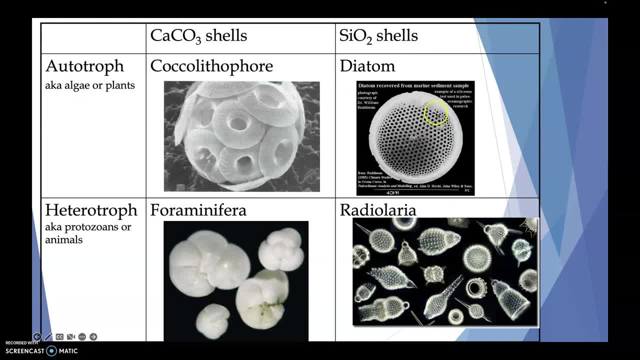 Are they made from an animal that makes its own food, or are they made of an animal that has to go and forage for its own food? So some ways that you may think of or some examples, I guess I should say, of some of these. 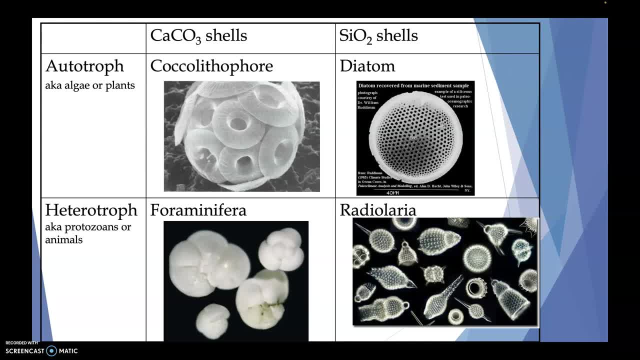 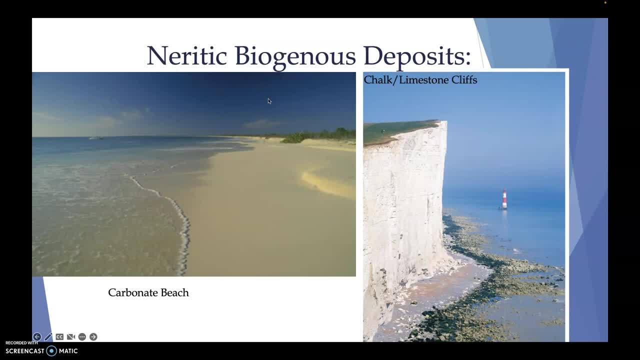 Creatures in sand form or in sediment form are the the neurotic biogenesis deposits. so I'm so sorry that I'm going to ruin any sort of beautiful sandy, fine sandy beach for you. but it turns out, a lot of those really beautiful tropical sandy beaches, even like the ones in Hawaii, are made up of fish poop. 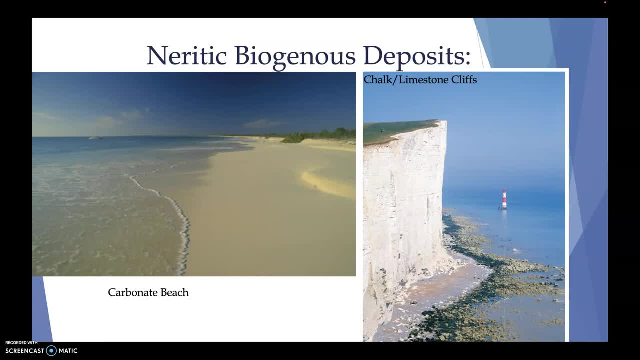 So fish poop, most specifically parrotfish, Eat coral and eat algae off of the coral and then they digest that coral and then their poop is then sand. So you're welcome. Sorry, but it's the truth. It's really quite fascinating. 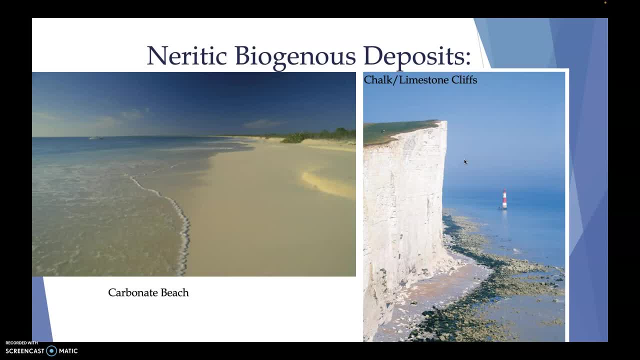 Or if you've ever had the opportunity to use chalkboards. the chalk that we use are actually old, old coccolithophores- Which, by the way, are my favorite plankton. They're just the most fun to say. but coccolithophores make up chalk or limestone cliffs. 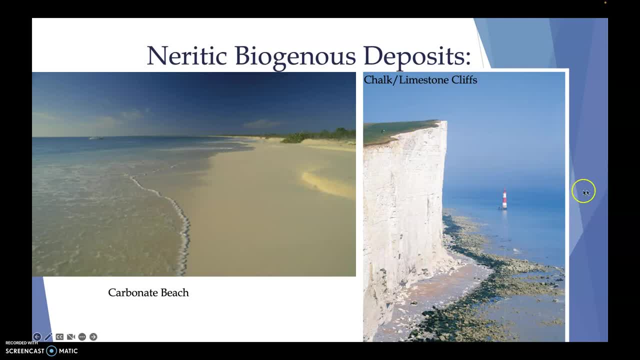 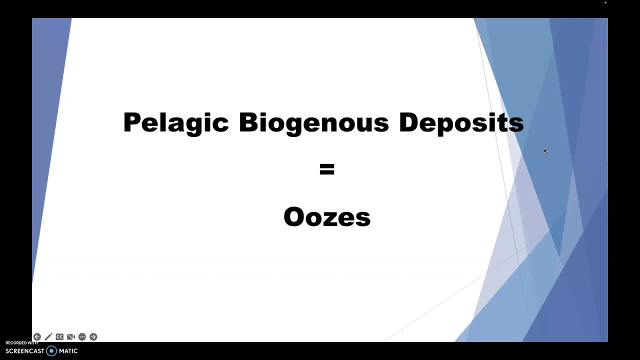 This is. these are limestone cliffs in England, So kind of cool. And then the last little bit in terms of biogenous sediments that I want to touch on are something called oozes, And this one's kind of weird. So these are pelagic biogenous deposits. 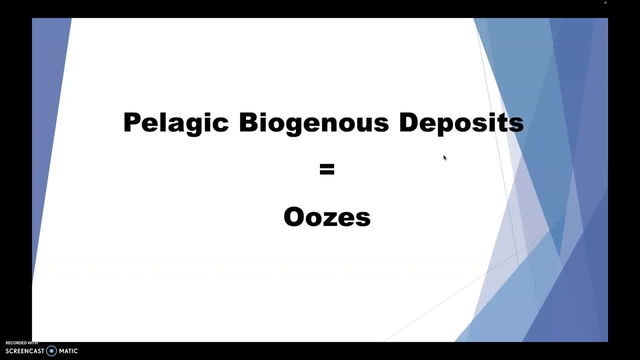 They're technically called oozes, But they're not like a sediment, They're like oozing out of- excuse me, of the bottom of the ocean. That's kind of a misconception, at least, that I had to break when I was learning about this. 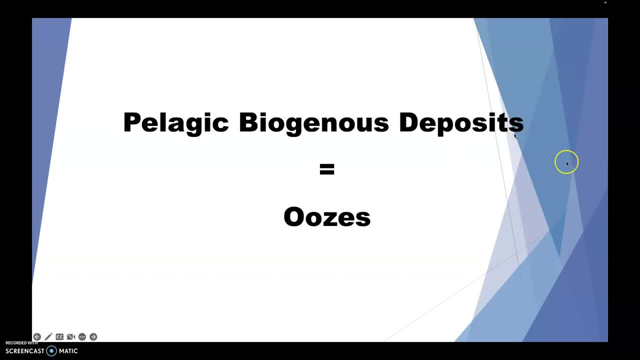 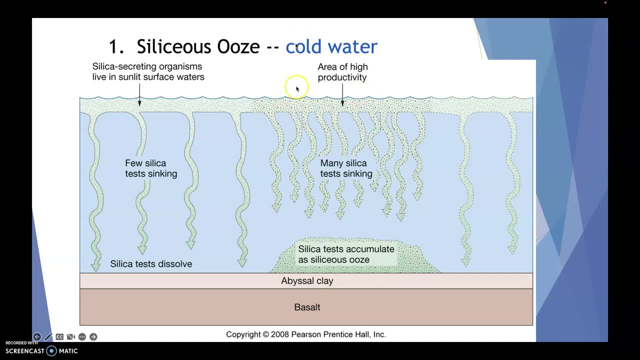 It's not like oozing out of the bottom, It's actually more so floating from from the top. There's two different kinds. The first is silica ooze, and that's generally found in colder waters. So in these, these cooler, cooler waters, here we have areas of higher productivity, meaning higher plankton blooms or higher plankton blooms.